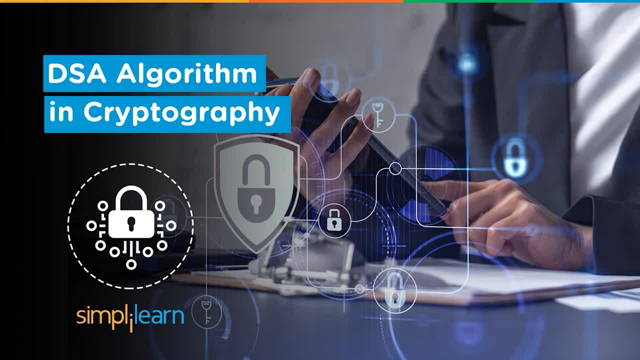 of scenarios. Thankfully, DSA algorithm has managed to solve this problem. The use cases for this cipher is rather niche, but crucial nonetheless. Let's take a look at the topics we need to cover in today's video. We first get a recap on what asymmetric encryption 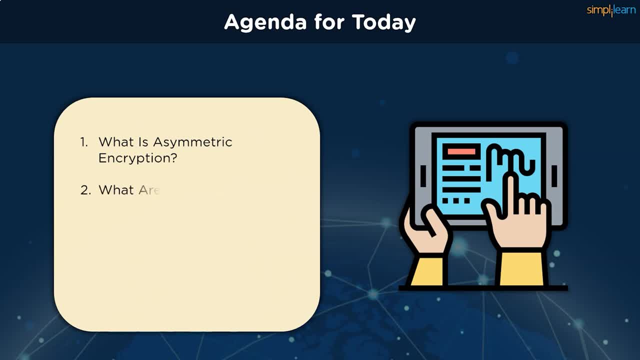 is and how is it any different from symmetric encryption? We learn what digital signatures are and how they are used in today's world. Next, we understand the digital signature algorithm and see how it works. Finally, we learn about the advantages DSA provides when it comes to managing digital 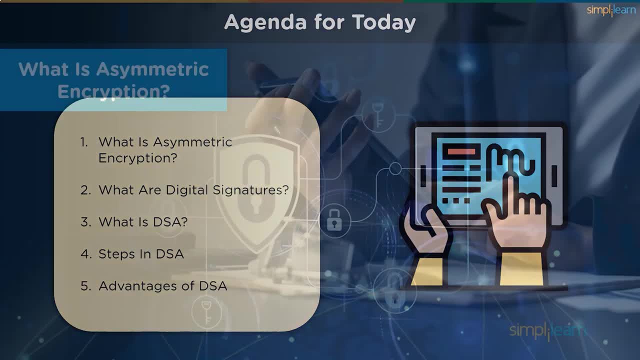 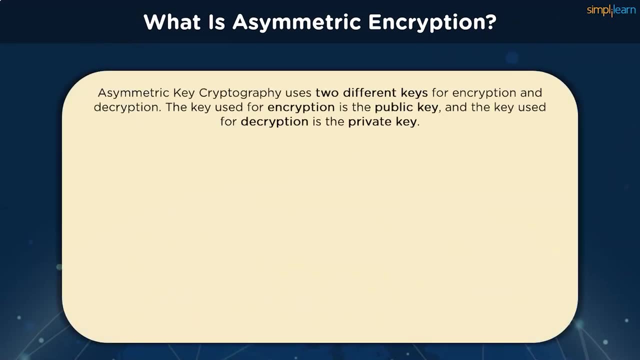 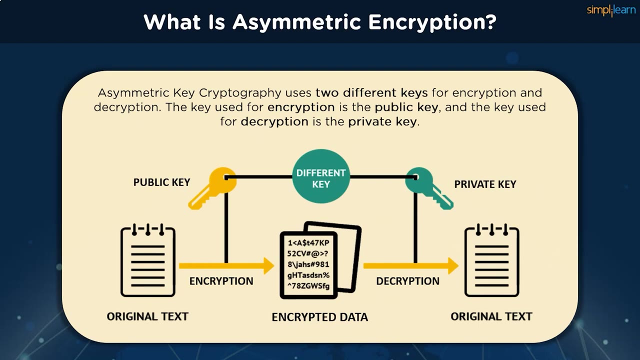 signatures in a corporate and a personal environment. Let's take a look at asymmetric encryption. Asymmetric encryption uses a double layer of protection. There are two different keys at play here: a private key and a public key. The public key is used to encrypt the information pre-transit and the private key is used to 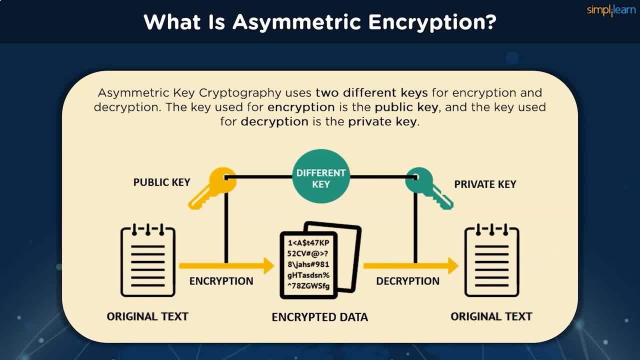 decrypt the data post-transit. This pair of keys must belong to the receiver of the message. The public keys can be shared via messaging, blog posts or key servers, since there are no restrictions. As you can see in the image, the two keys work in the system. 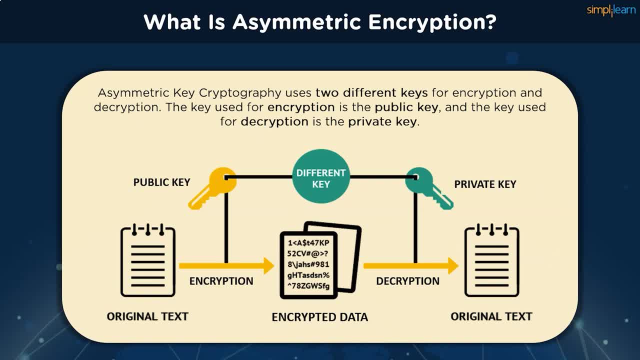 The sender first encrypts the message using the receiver's private key, after which we receive the ciphertext. The ciphertext is then transmitted to the receiver without any other key. On getting the ciphertext, the receiver can use his or her own private key to decrypt the information and get the clear text back. 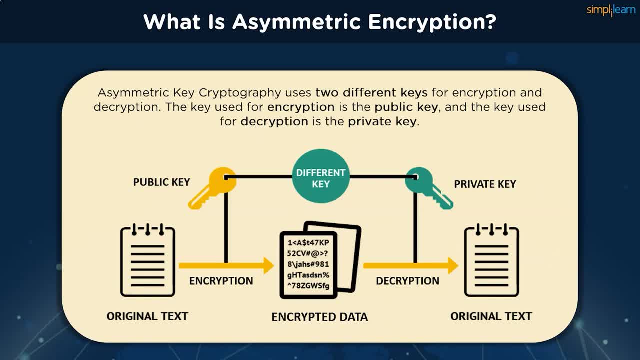 There has been no requirement of any key exchange throughout this process, therefore solving the most glaring flaw faced in asymmetric key cryptography. The public key known to everyone cannot be used to decrypt messages, and the private key which can decrypt messages need not be shared with anyone. The sender and receiver can exchange. 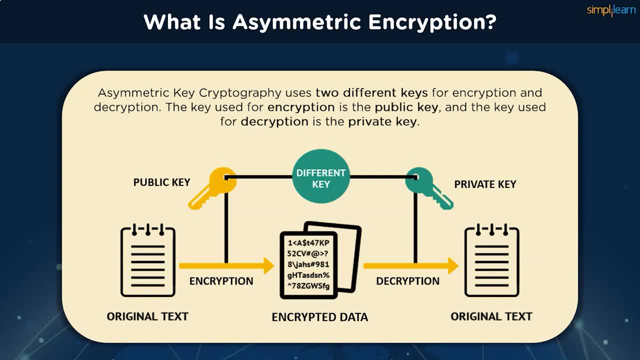 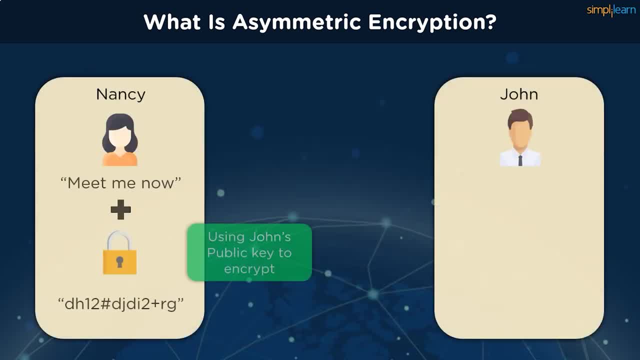 personal data using the same set of keys for as often, as long as possible. In this example, we have two people, Nancy and John. If Nancy wants to send a message to John, John's public key should be used to encrypt the information, The ciphertext. 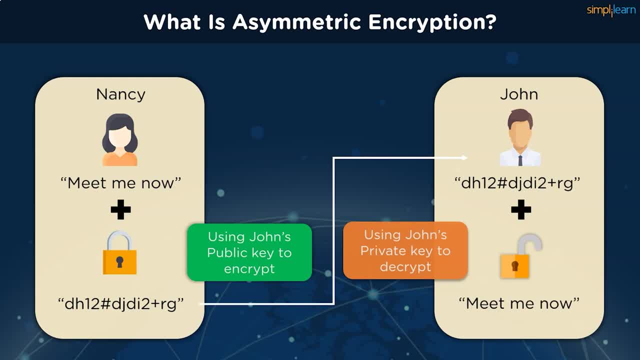 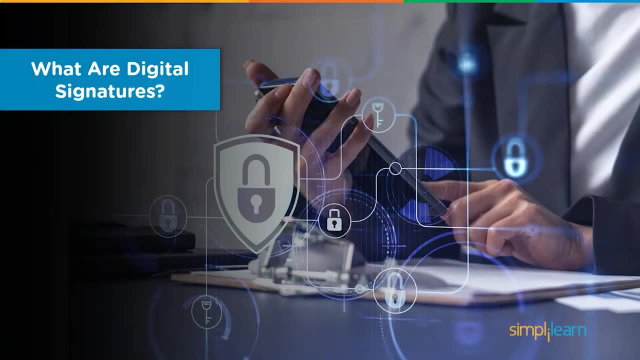 is then transferred to John, who can use his private key to decrypt the data and get the plain text back. This goes to highlight how we have overcome the problem of key sharing when it comes to asymmetric encryption. Now that we have a proper revision, let's 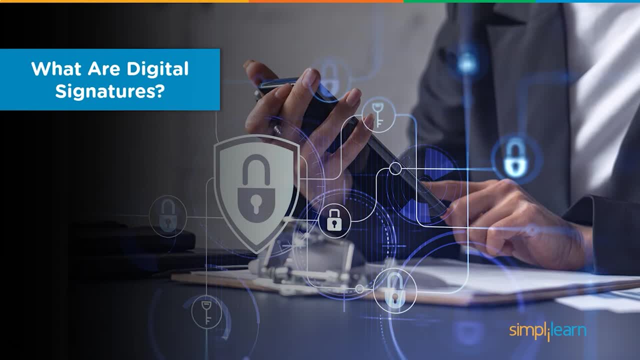 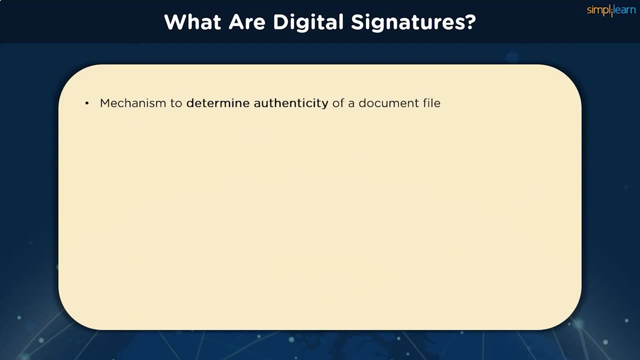 understand what digital signatures are before moving on to the algorithm. The objective of digital signatures is to authenticate and verify documents and data. This is necessary to avoid tampering and digital modification or forgery of any kind during the transmission of official documents. They work on the public key cryptography architecture. 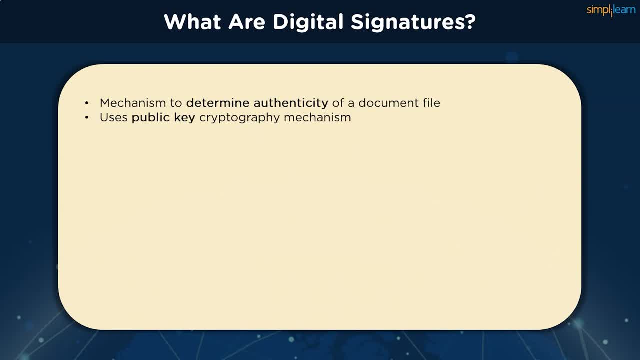 with one exception. Typically, an asymmetric key system encrypts using a public key and decrypts the information. The system is then used to decrypt messages and messages to the private key. For digital signatures, however, the reverse is true: The signature is encrypted. 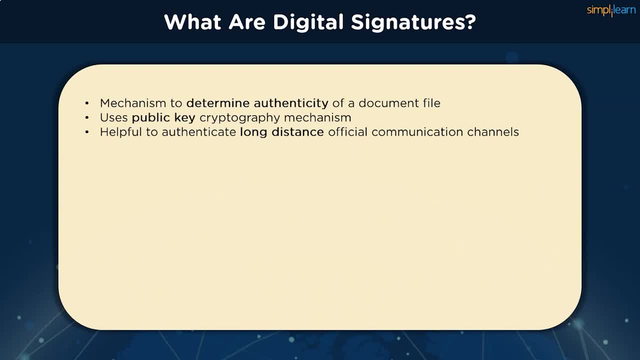 using a private key and is decrypted with the public key, Because the keys are inked together. decoding it with the public key verifies that the proper private key was used to sign the document, thereby verifying the signature's provenance. Let's go through. 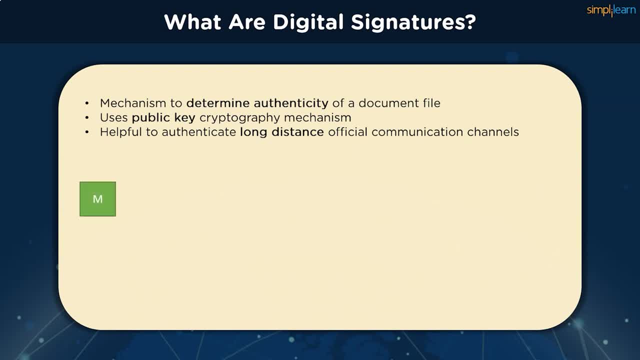 each step to understand the procedure thoroughly. In step 1, we have M, which is the original plain text message, And it is passed onto a hash function denoted by H- hash, to create a digest. Next, it bundles the message together with the hash digest and encrypts it using the 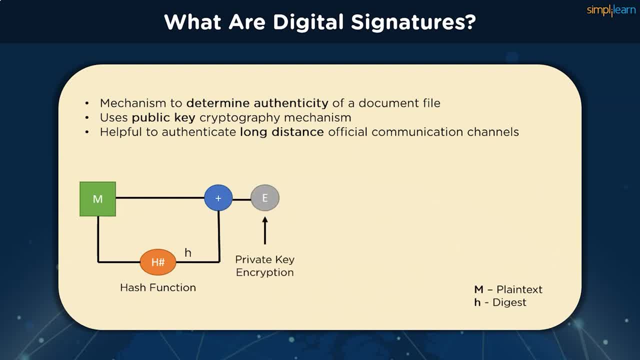 sender's private key. It sends the encrypted bundle to the receiver, who can decrypt it using the sender's public key. Once the message is decrypted, it is passed through the same hash function- H hash- to the sender's private key. Once the message is decrypted, it is passed. 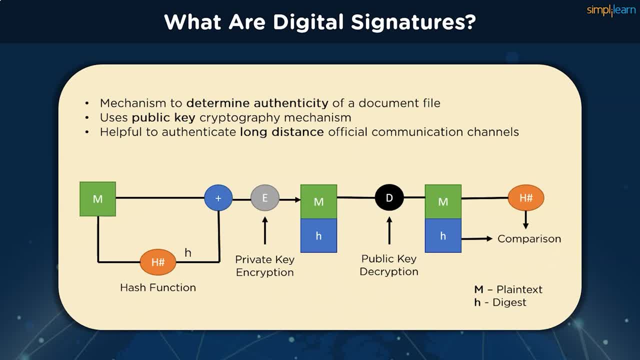 through the same hash function and encrypts it using the sender's private key. And once the message is decrypted, it is passed through the same hash function- H hash- to the sender's private key. Next, we have a new hash function called the hash divider. It is used to create a similar 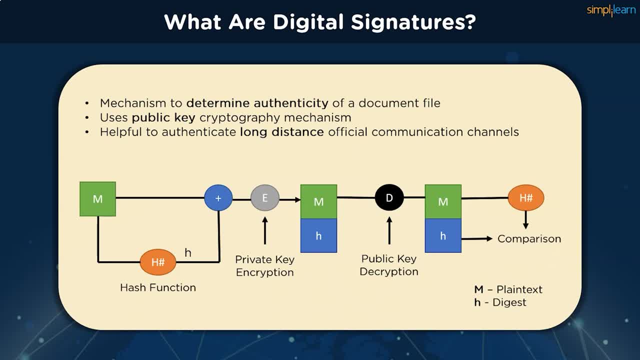 digest. It compares the newly generated hash with the bundled hash value received, along with the message. If they match, it verifies data integrity. In many instances, they provide a layer of validation and security to messages through a non-secured channel, Properly implemented. 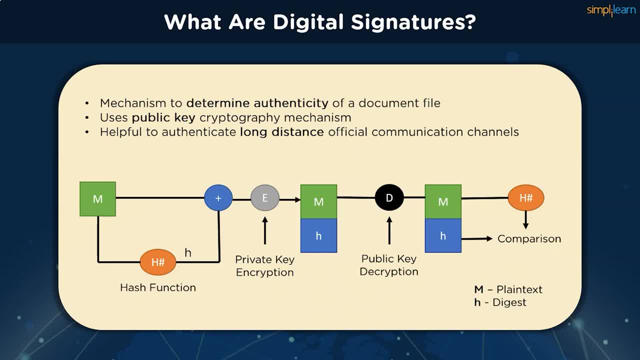 a digital signature gives the receiver reason to believe that the message was sent by the claimed sender. Digital signatures are equivalent to traditional handwritten signatures in a many respects, but properly implemented digital signatures are more difficult to forge than the handwritten type. Digital signature schemes, in the sense used here, are cryptographically based and must. 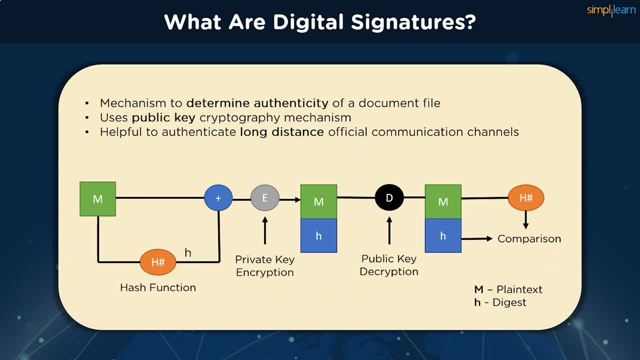 be implemented properly to be effective. They can also provide non-repudiation, meaning that the signer cannot successfully claim that they did not sign a message while also claiming their private key remains secret. Further, some non-repudiation schemes offer a timestamp for the digital signature, so 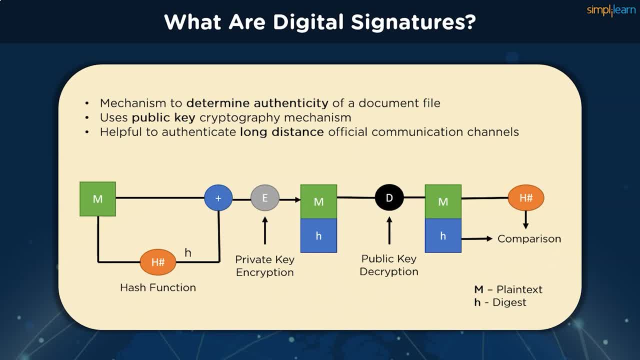 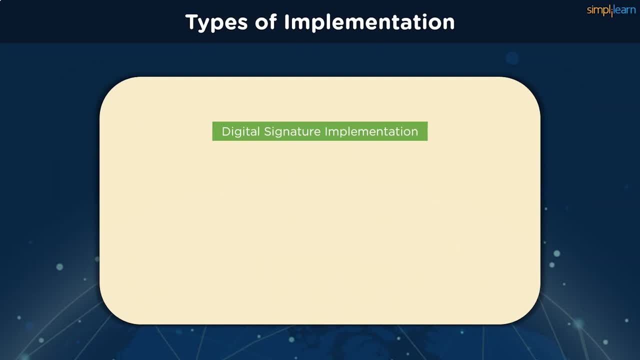 that, even if the private key is exposed, the signature is valid. To implement the concept of digital signature in real world, we have two primary algorithms to follow: the RSA algorithm and the DSA algorithm, but the latter is a topic of learning today. 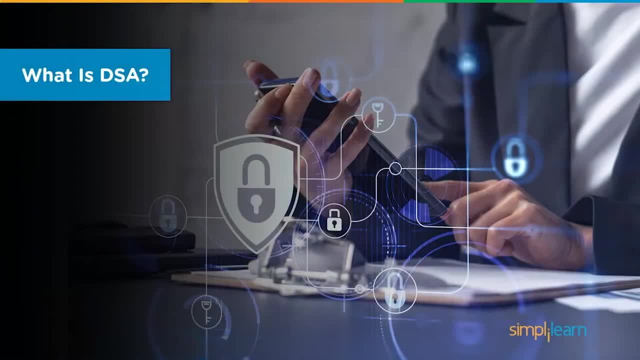 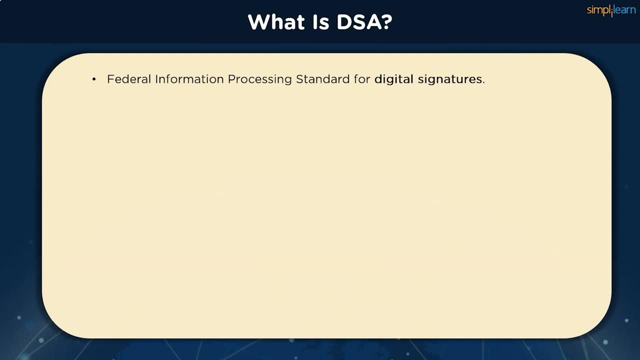 So let's go ahead and see what the digital signature algorithm is supposed to do. Digital signature algorithm is a FIPS standard, which is a Federal Information Processing Standard. It was proposed in 1991 and globally standardized in 1994 by the National Institute of Standards. 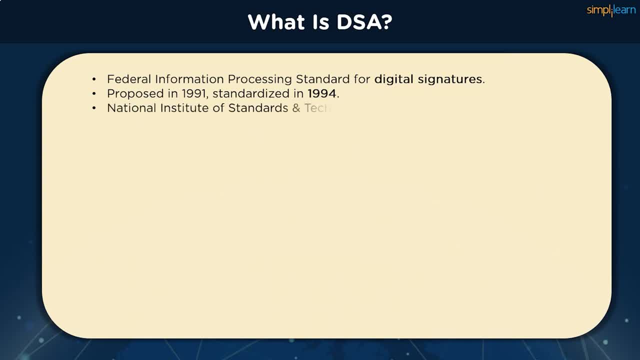 and Technology. It functions on the framework of modular exponention and discrete logarithmic problems which are difficult to compute as a force-brood system. Unlike DSA, most signature types are generated by signing message digests with the private key of the originator. 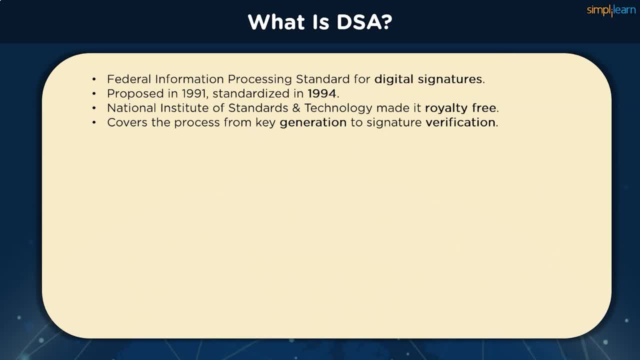 This creates a digital thumbprint of the data. Since just the message digest is signed, the signature is generally much smaller compared to the data that was signed. As a result, digital signatures impose less load on processors at the time of signing execution and they use small volumes of bandwidth. 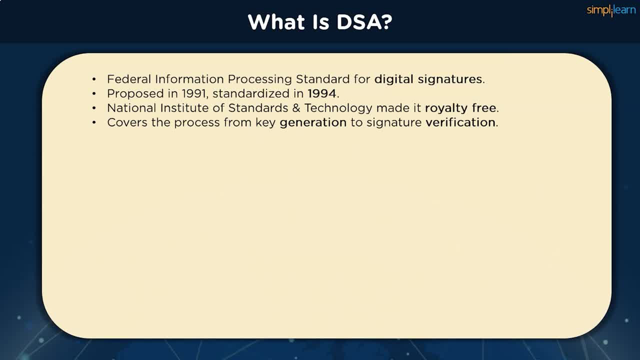 DSA, on the other hand, does not encrypt message digests using private key or decrypt message digests using public key. Instead, it uses mathematical functions to create a digital signature consisting of two 160-bit numbers, which are originated from the message digests and the private key. 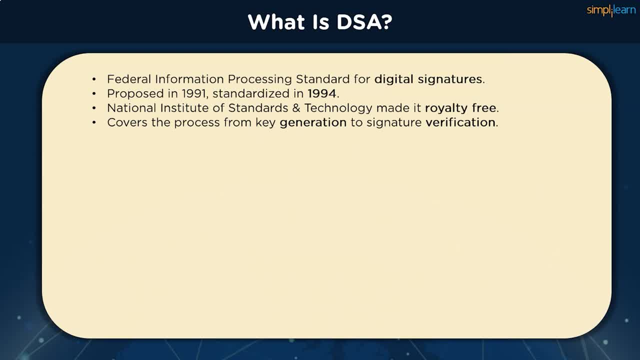 DSAs make use of the public key for authenticating the signature, but the authorization process is much more complicated when compared with RSA. DSA also provides three benefits, which is the message: authentication, integrity, verification and non-repudiation. In the image, we can see the entire process of DSA validation. 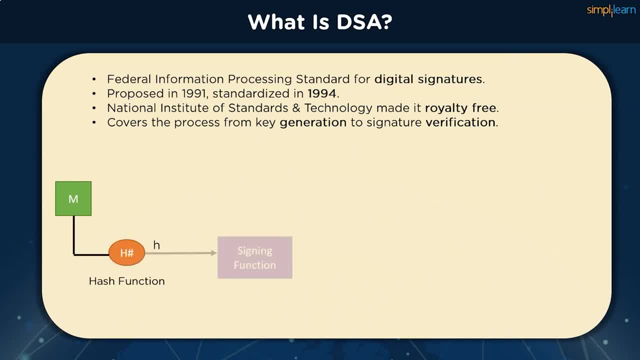 A plain text message is passed onto a hash function Where the digest is generated, which is passed onto a signing function. Signing function also has other parameters, like a global variable G, a random variable K and the private key of the sender. The outputs are then bundled onto a single pack with the plain text and sent to the receiver. 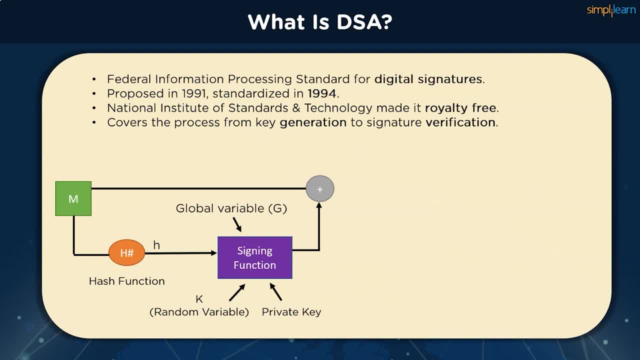 The two outputs we receive from the signing functions are the two 160-bit numbers denoted by S and R. On the receiver end we pass the plain text to the same hash function to regenerate the message digest. It is passed onto verification function, which has other requirements such as the public. 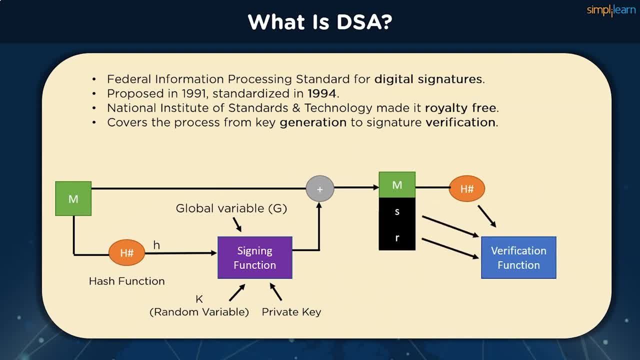 key of the sender global variable G and S and R received from the sender. The value generated by the function is then compared to R. If they match, then the verification process is complete and data integrity is verified. This was an overview of the way the DSAs work. 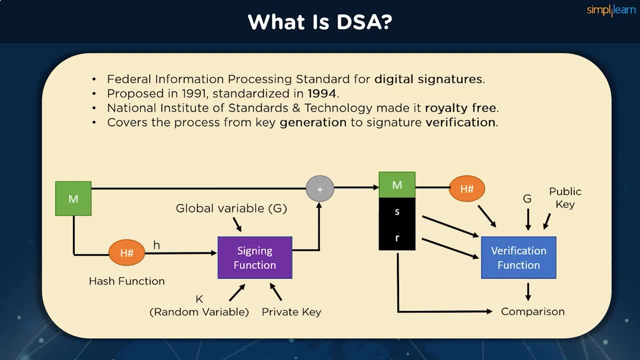 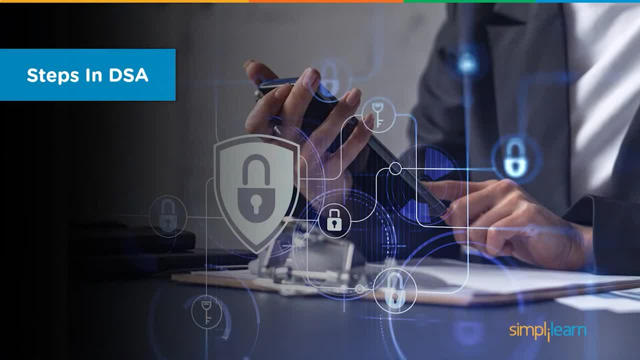 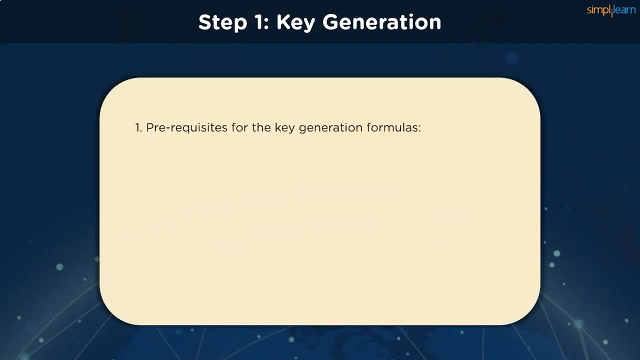 We already know it depends on logarithmic functions to calculate the outputs, So let us see how we can do the same in our next section. We have three phases here, The first of which is key generation. To generate the keys, we need some prerequisites. 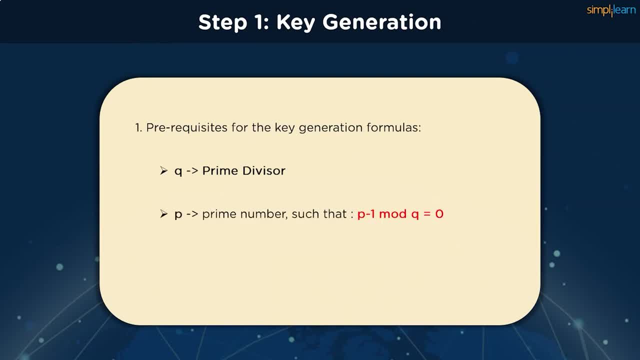 We'd select a Q, which becomes a prime divisor. We select a prime number, P, such that P-1 mod Q equal to zero. We also select a random integer G. This satisfies the two formulas being mentioned on the screen right now. Once these values are selected, we can go ahead with generating the keys. 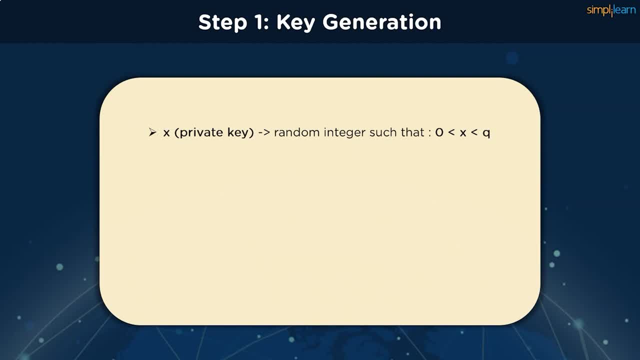 The private key can be denoted by X and it is any random integer that falls between the bracket of zero and the value of Q. The public key can be calculated as Y equal to G to the power X mod P, where Y stands for the public key. 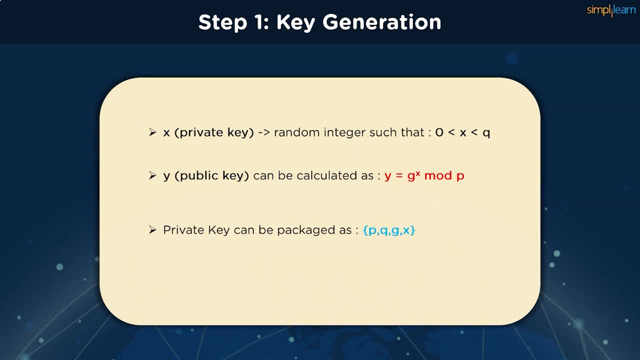 The private key can then be packaged as a bundle Which comprises of Values of P, Q, G and X. Similarly, the public key can also be packaged as a bundle having the values of P, Q, G and Y. Once we're done with key generation, we can start verifying the signature and its generation. 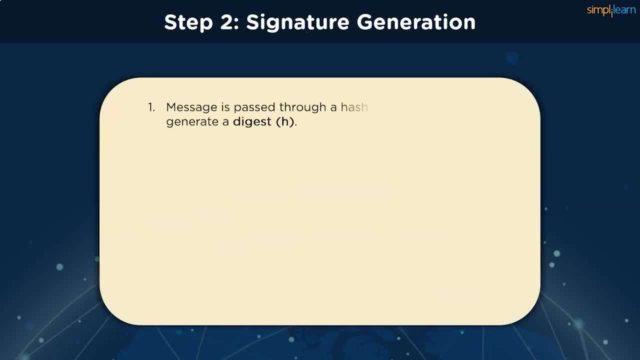 Once the keys are generated, we can start generating the signature. The message is passed through a hash function to generate the digest edge first. Please remember the segundaub. lay it off withлушай future lawyers. So at the end of the playday we've directed the first. establish a sweety for validating. 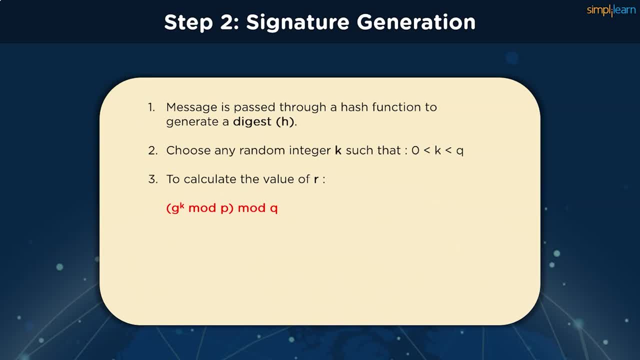 the signature. if you cannot practically use the signature and persistent mm By using the formula G to the power K, bind p- 17,. into mod Q goes that Q and this is the case in the case of C, And each is read as a seed. 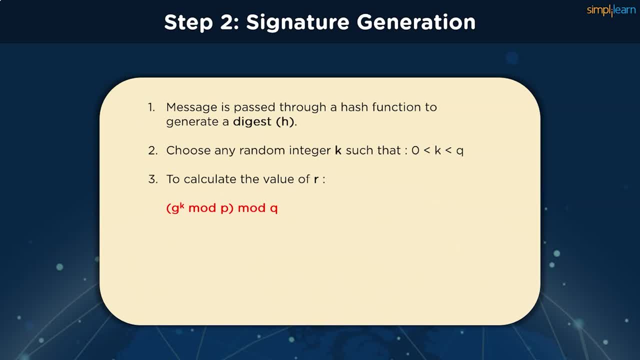 This is an operator, toisfilium, and they just says VAD as well, Milk. In other other words, with this representation, we can Ingredients. there are passes between the at error period of the objects, with or without a delay for the so forth. Similarly, if the fils is at error or with or without a delay, or anytime the addition load, we need to take out the very females there in the field. We'll see about that at a later green screen right now where Vs were separate from. 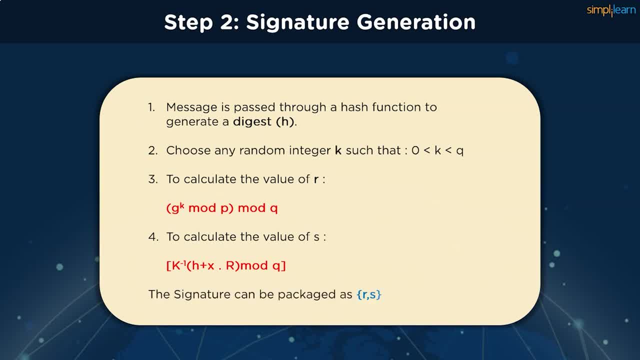 We use the following formula that is shown on the screen. The signature can then be packaged as a bundle having R and S. This bundle, along with the plain text message, is then passed on to the receiver. Now, with the third phase, we have to verify the signature. 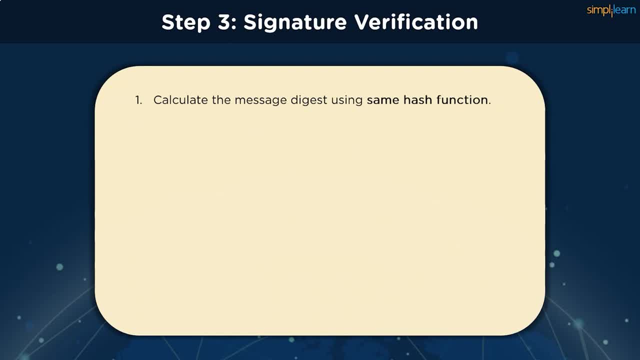 We first calculate the message digest received in the bundle by passing it to the same hash function. We calculate the value of W, U1 and U2 using the formulas shown on the screen. We have to calculate a verification component which is then to be compared with the value. 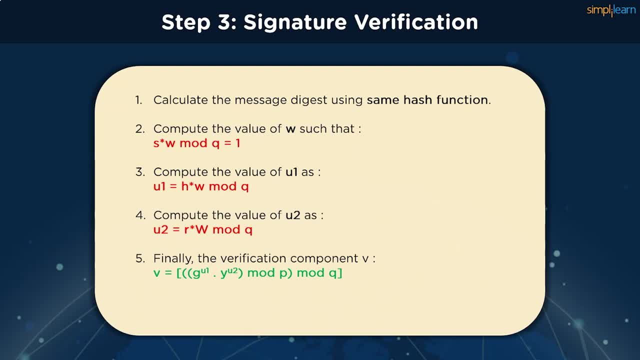 of R being sent by the sender. This verification component can be calculated using the following formula: Once calculated, this can be compared with the value of R. If the values match, then the signature verification is successful and the entire process is complete, starting from. 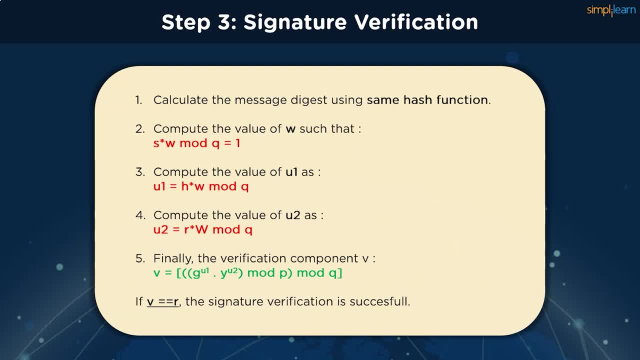 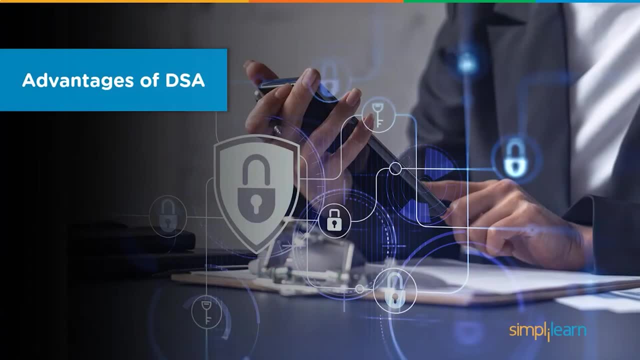 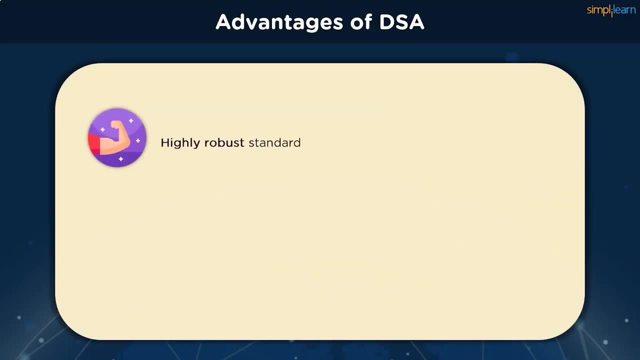 key generation to the signature generation, all the way up to the verification of the signature. With so many steps to follow, we are bound to have a few advantages to boot this, and we would be right to think so. DSA is highly robust in the security and stability aspect when compared to alternative signature.